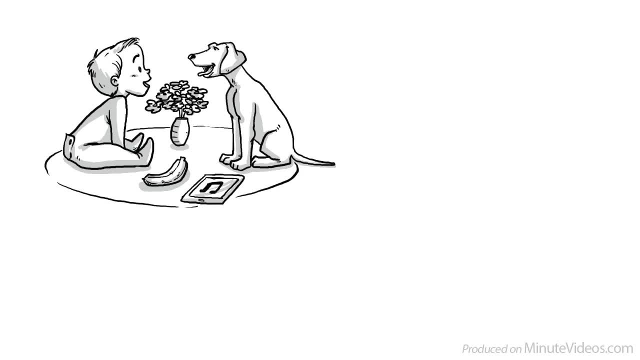 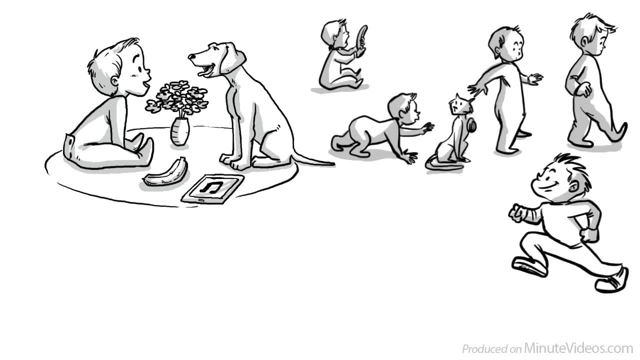 sounds and talk to strangers, To explore more. we move, We learn to sit, crawl, stand, walk and even to run. This increased physical mobility consequently leads to increased cognitive development. But we remain egocentric, meaning we can. 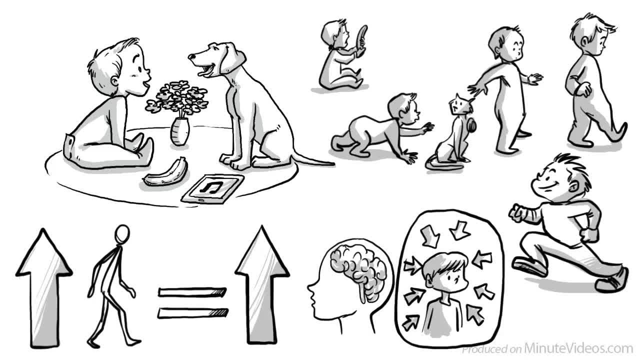 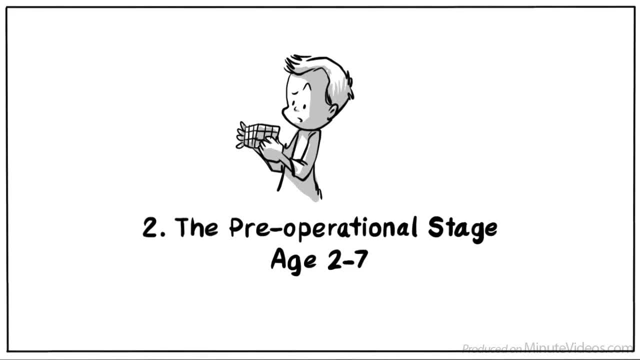 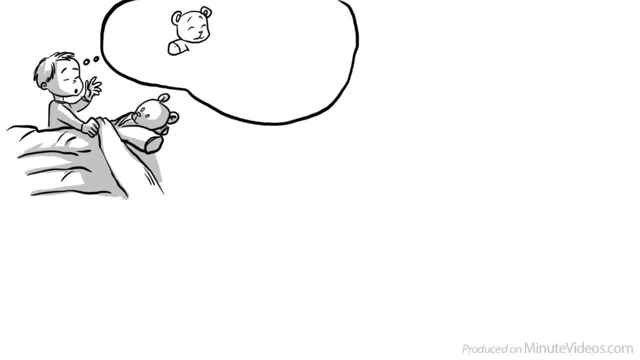 perceive the world only from our own point of view. The pre-operational stage ages 2 to 7. Our thinking is mainly categorized through symbolic functions and intuitive thoughts. We have lots of fantasies and believe objects are alive, As we are not able to apply specific cognitive operations- Piaget calls this. 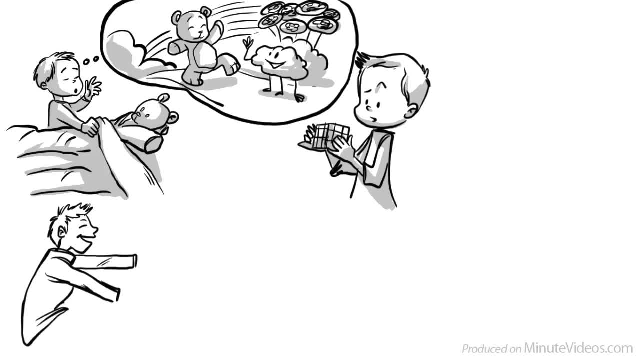 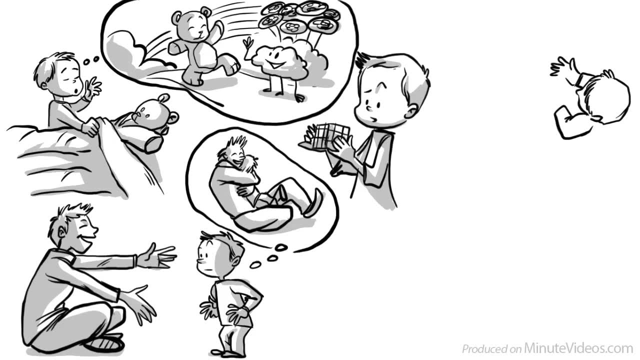 stage, pre-operational, We learn to speak and understand that words, images and gestures are symbols for something else. When we draw our family, we are not concerned about drawing each person to scale, but rather with their symbolic meanings. We love to play pretend, which allows us. 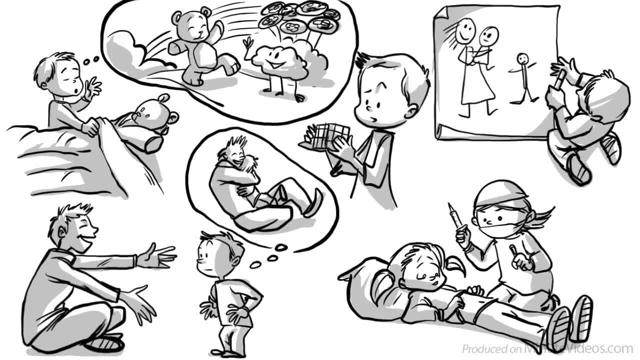 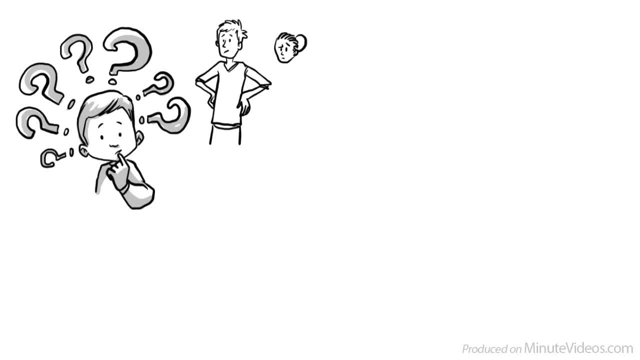 to experience something new and learn a lot. At around age 4,, most of us become very curious and ask many questions. We want to know everything. We can call it the bird's birth of primitive reasoning. Piaget calls it the intuitive age, because, while we realize, 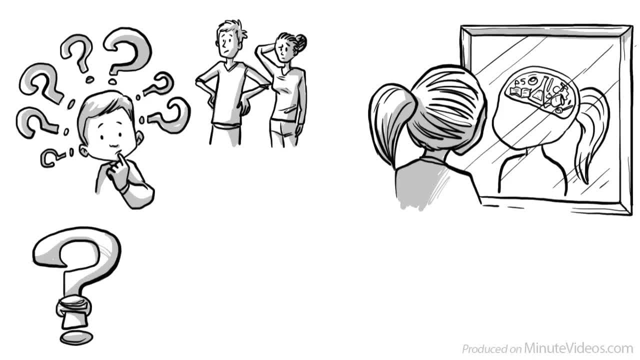 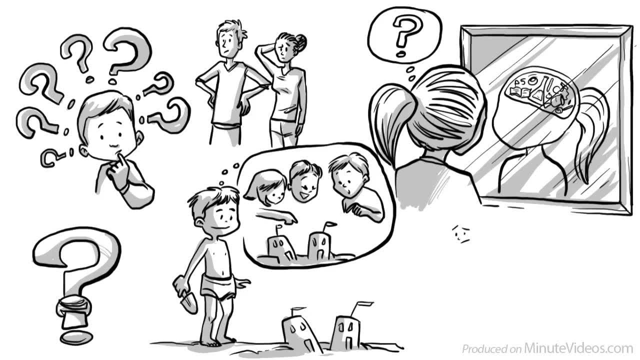 that we have a vast amount of knowledge. we have no idea how we acquired it. Our thinking in this stage is still pretty egocentric. We think others see the world like we do and still don't understand that they see it differently. 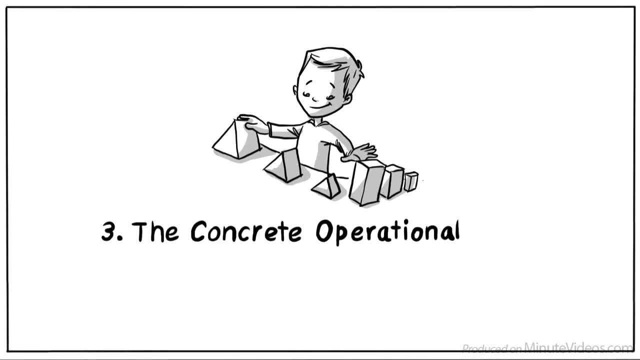 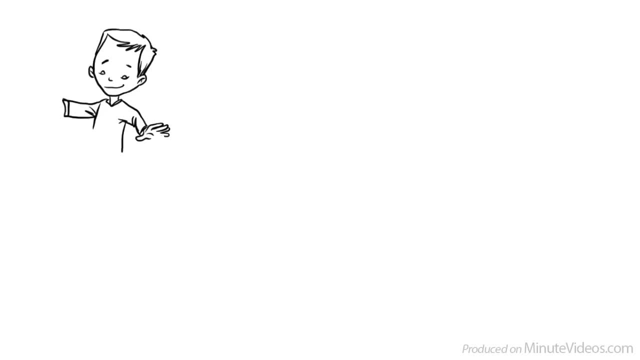 3. The concrete operational stage ages 7 to 11. We finally discover logic and we develop concrete cognitive operations such as sorting objects in a certain order. One example of this is inductive reasoning, which means that if we see someone eating a cookie, we can draw a conclusion and then make a generalization. 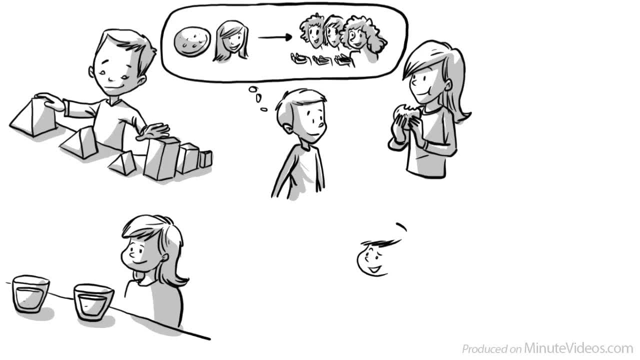 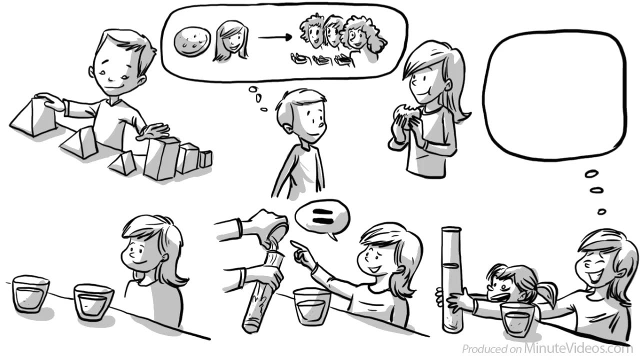 And we now get the concept of conservation. We understand that if we pour orange juice from a normal glass to a taller one, the amount stays the same. Our younger sister will pick the taller glass, thinking she gets more. By the same logic we only now can understand. 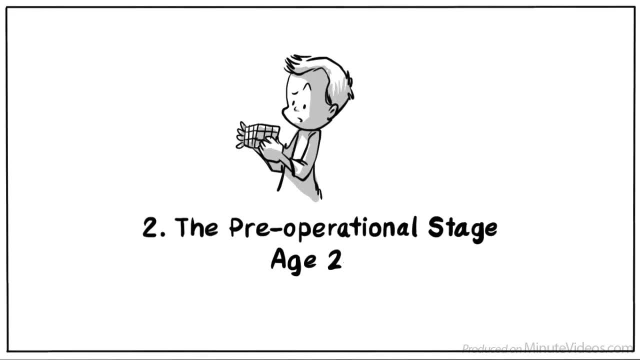 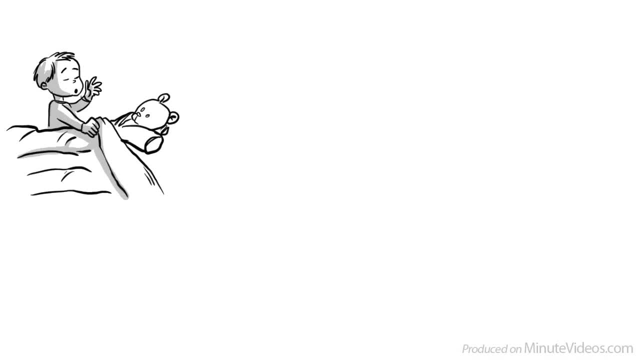 2. The pre-operational stage- ages 2 to 7. Our thinking is mainly categorized through symbolic functions and intuitive thoughts. We have lots of fantasies and believe objects are alive. As we are not able to apply specific cognitive operations, Piaget calls this stage pre-operational. 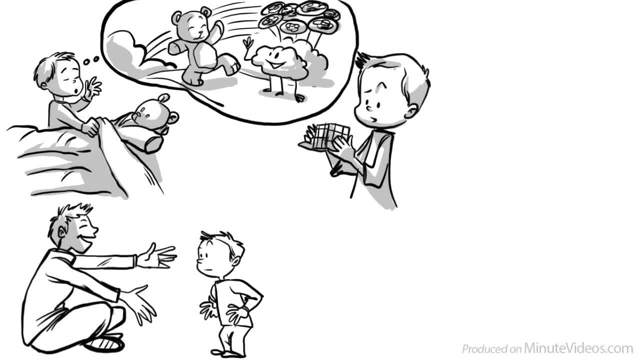 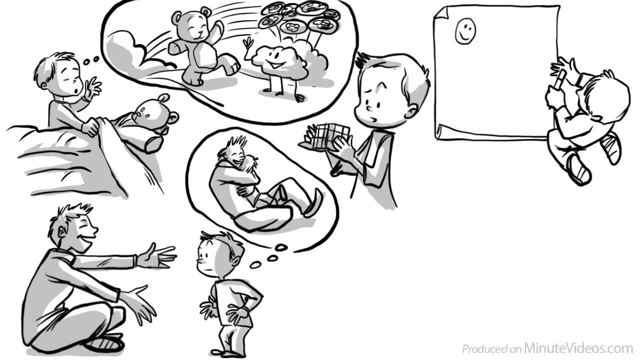 We learn to speak and understand that words, images and gestures are symbols for something else. When we draw our family, we are not concerned about drawing each person to scale, but rather with their symbolic meanings. We love to play pretend, which allows us to experience something new and learn a lot. 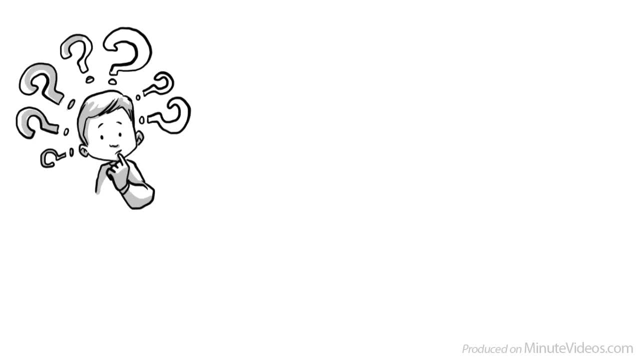 At around age 4, most of us become very curious and ask many questions. We want to know everything. We can call it the birth of primitive reasoning. Piaget calls it the intuitive age Because, while we realize that we have a vast amount of knowledge, 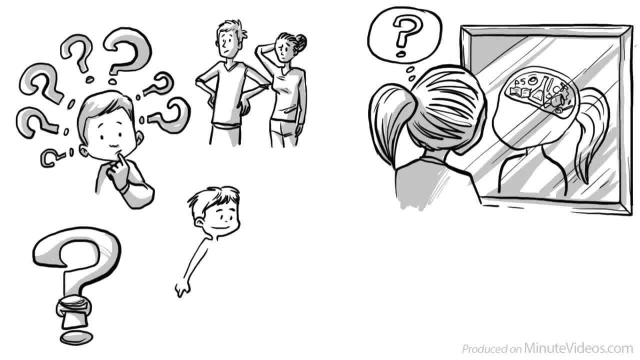 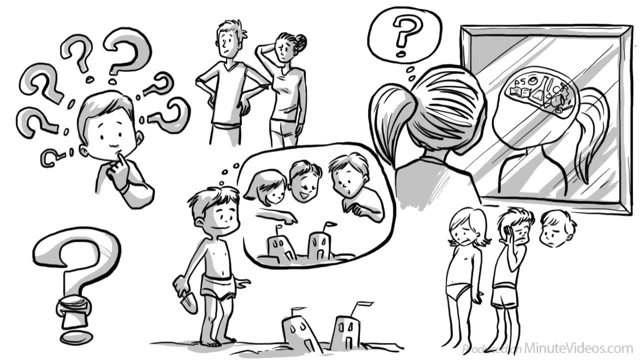 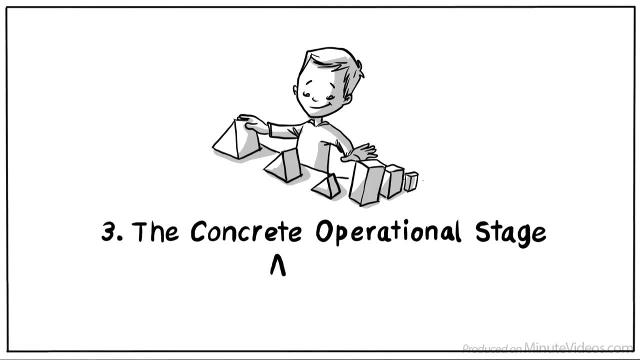 we have no idea how we acquired it. Our thinking in this stage is still pretty egocentric. We think others see the world like we do and still don't understand that they see it differently. 3. The concrete operational stage: ages 7 to 11. 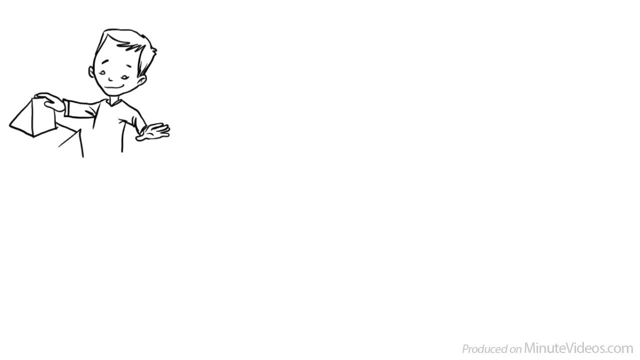 We finally discover logic and we develop concrete cognitive operations which allow us to understand what we are doing and what we are not doing. We can now understand that we are creating objects in a certain order. One example of this is inductive reasoning, which means that if we see someone eating a cookie, 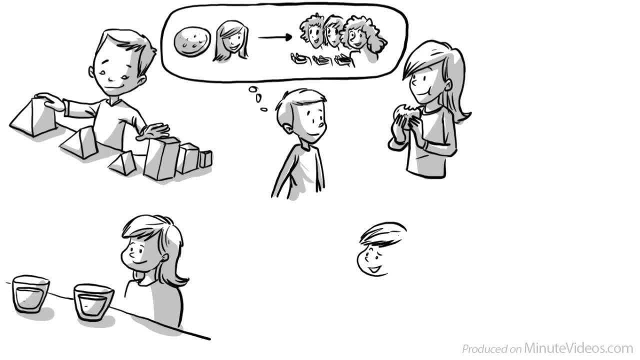 we can draw a conclusion and then make a generalization And we now get the concept of conservation. We understand that if we pour orange juice from a normal glass to a taller one, the amount stays the same. Our younger sister will pick the taller glass, thinking she gets more. 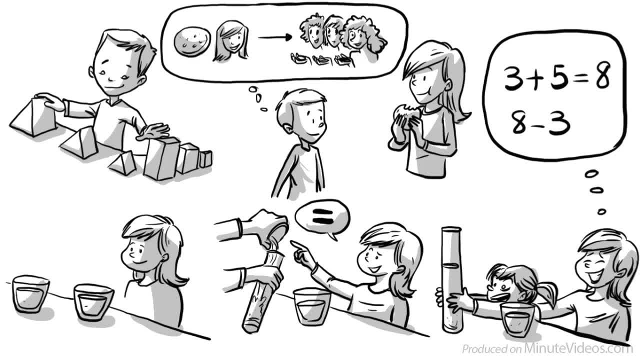 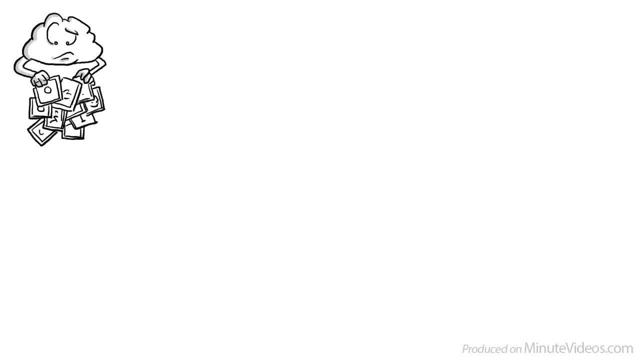 We can now understand that if 3 plus 5 equals 8, then 8 minus 3 must equal 5.. Our brain learns to rearrange our thoughts, to classify and build concrete operational mental structures. For example, we now know that we can reverse an action by doing the opposite. 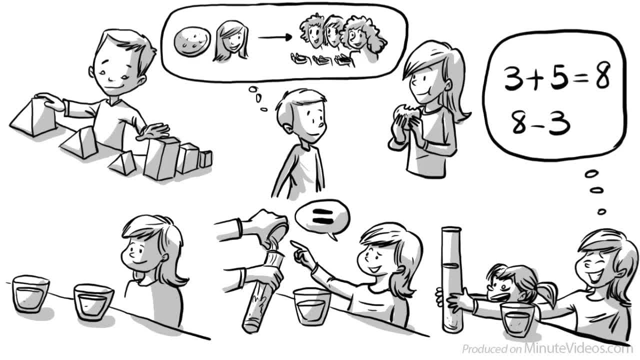 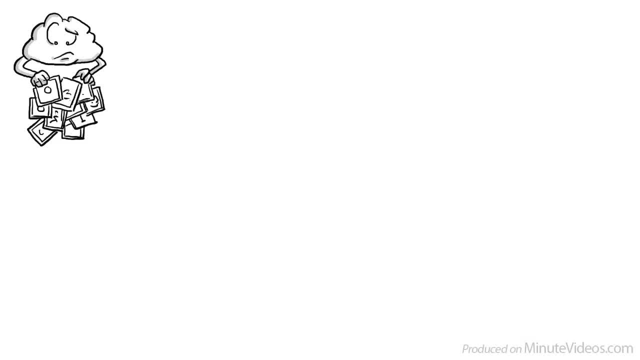 that if 3 plus 5 equals 8, then 8 minus 3 must equal 5.. 4. The state of mind: Our brain learns to rearrange our thoughts, to classify and build concrete operational mental structures. For example, we now know: 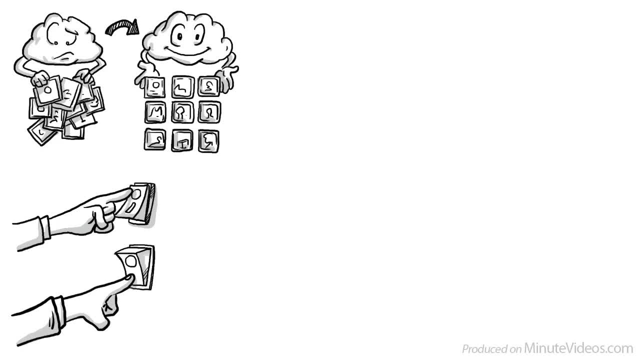 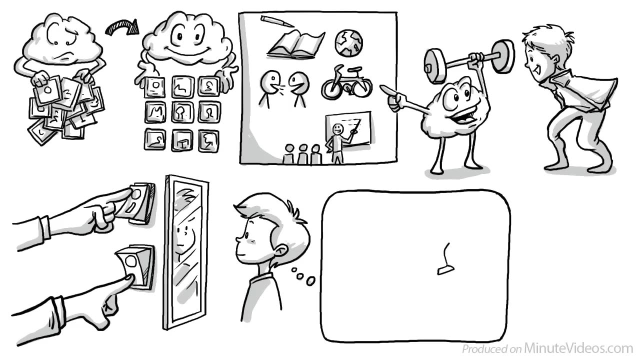 that we can reverse an action by doing the opposite. Excited by our new mental abilities, We apply them in conversations, activities, when we learn to write, and in school. As a result, we get to know ourselves better. We begin to understand that our thoughts and feelings are unique, and not necessarily those. 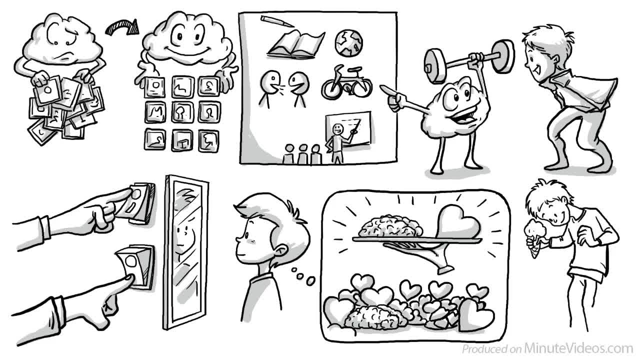 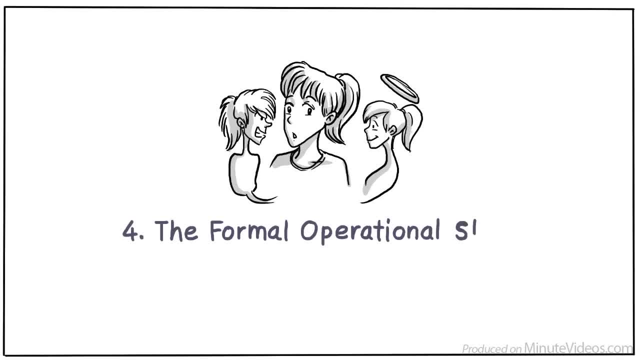 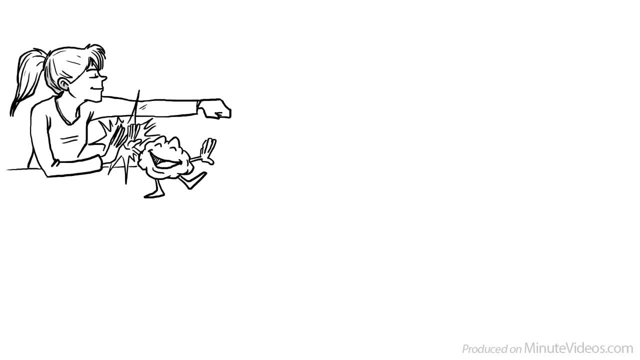 of others. That means that we learn to put ourselves in someone else's shoes. 4. The Formal Operational Stage. As we become teenagers, we become formally operational. We now have the ability to think more rationally about abstract concepts and hypothetical events. 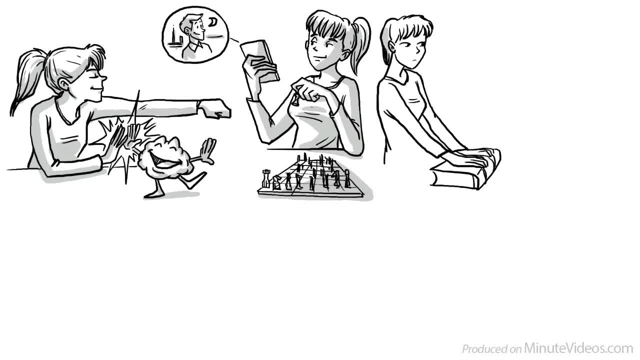 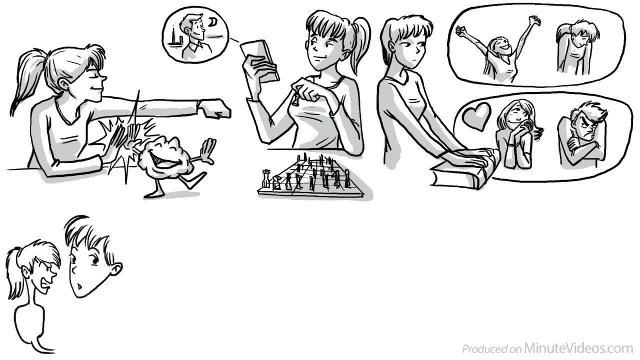 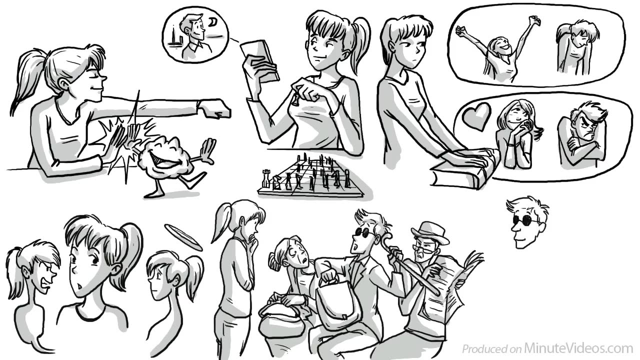 Our advanced cognitive abilities allow us to understand abstract concepts such as success and failure, love and hate. We form a deeper understanding of our own identity and our morality. We now also think that we understand why people behave the way they behave and, as a result, 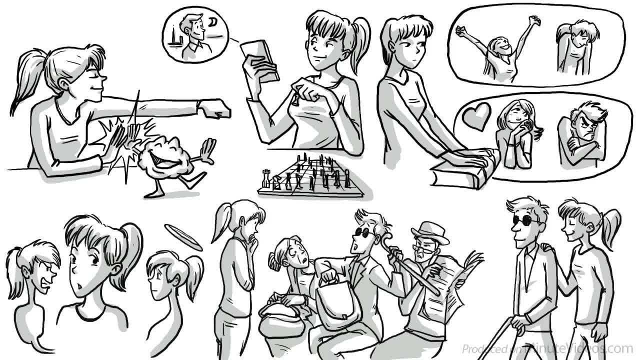 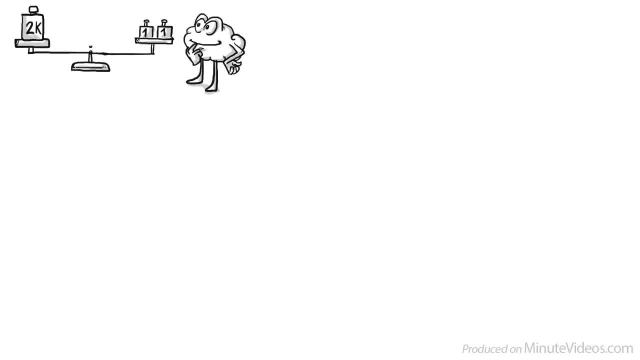 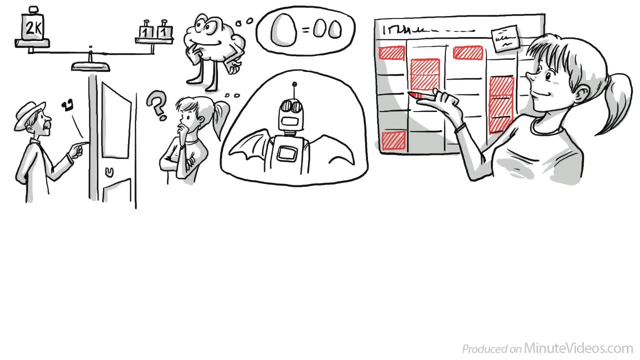 we can become more compassionate. Our brain can now do deductive reasoning, which means we can compare two statements and reach a logical generalization. Our new mental skills allow us to plan our life systematically and prioritize, And we can make assumptions about events that have no necessary relation to reality. 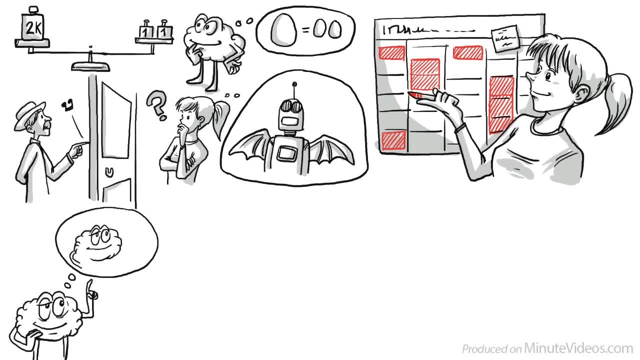 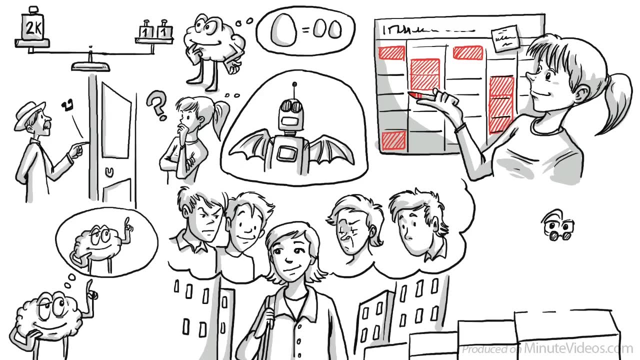 We can now also philosophize and just think about thinking itself. Our new sense for our identity now also creates egocentric thoughts, and some start to see an imaginary audience watching them all the time. Piaget believed in lifelong learning, but insisted that the formal, operational stage 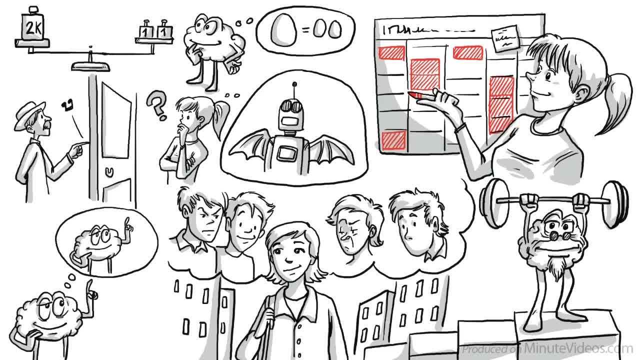 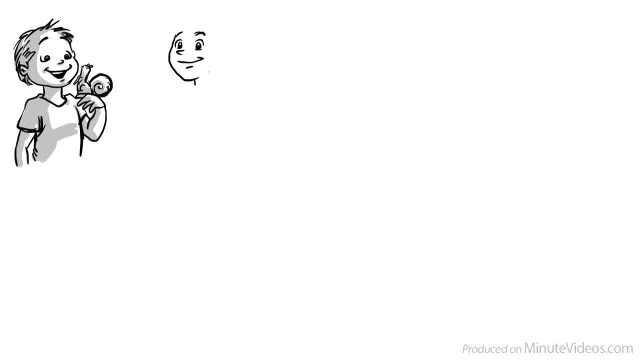 is the final stage of our cognitive development. 4. The Scientific Fragment. Jean Piaget's first interests were animals and he published his first scientific paper on albino sparrows in 1907.. 5. when he was just 11 years old. 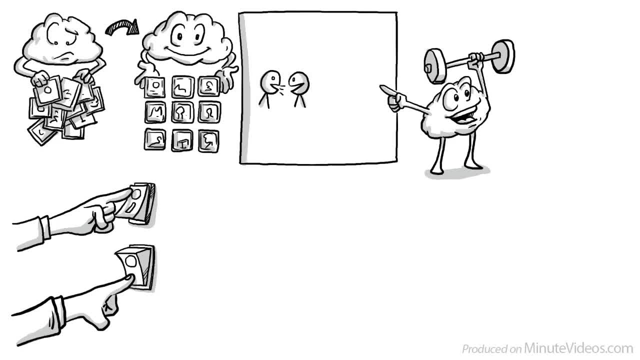 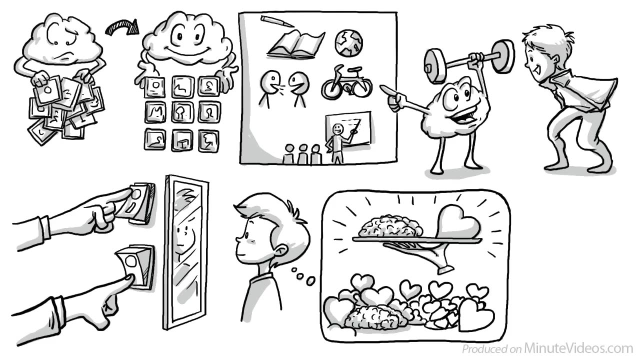 Excited by our new mental abilities, we apply them in conversations, activities, when we learn to write, and in school. As a result, we get to know ourselves better. We begin to understand that our thoughts and feelings are unique and not necessarily those of others. That means that we learn to put ourselves. 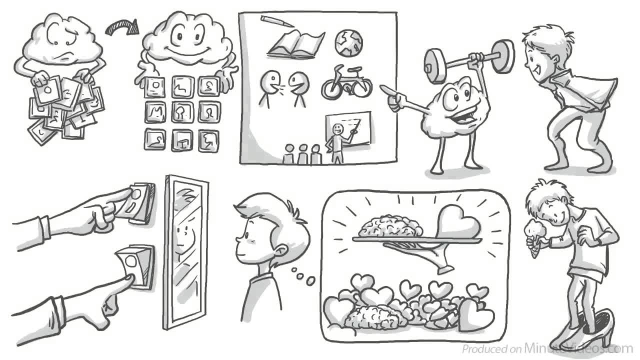 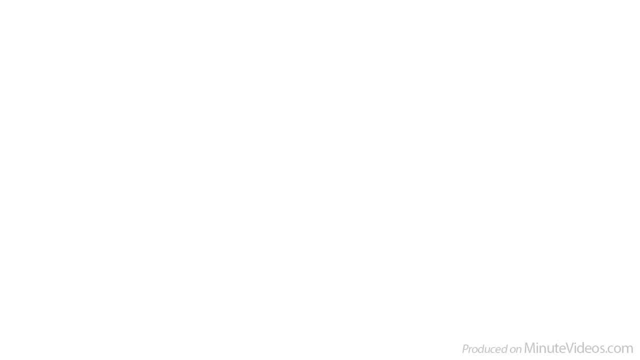 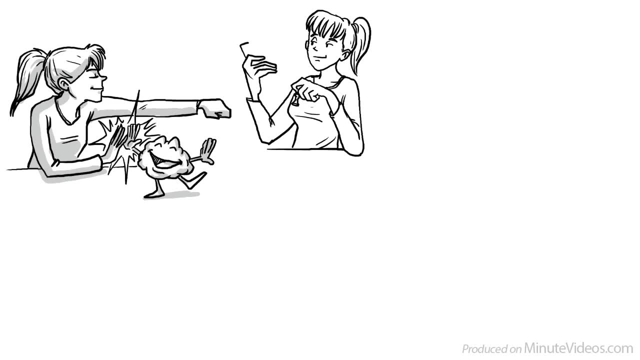 in someone else's shoes. 4. The Formal Operational Stage. Once we become teenagers, we become formally operational. We now have the ability to think rationally about abstract concepts and hypothetical events. Our advanced cognitive abilities allow us to understand abstract concepts such as success. 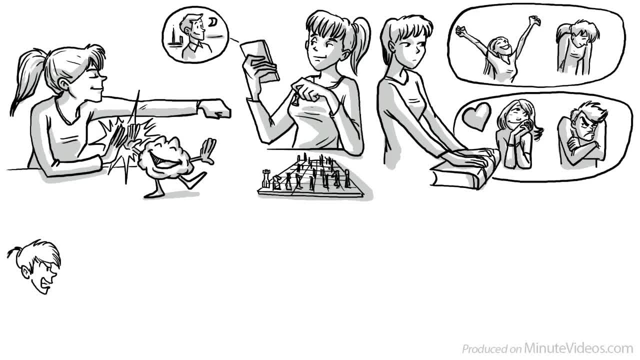 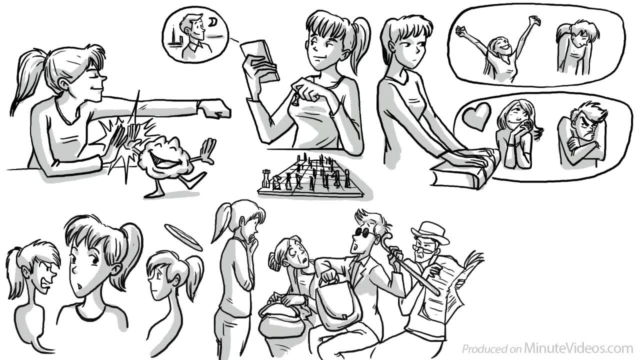 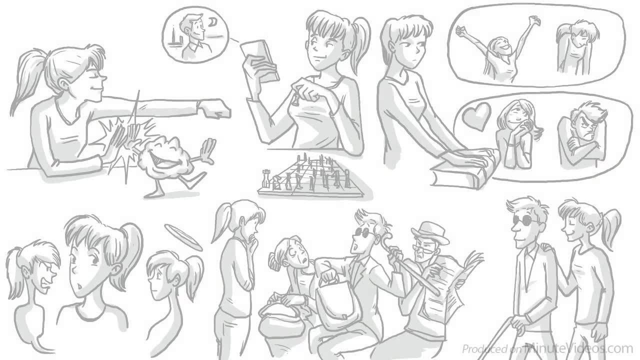 and failure, love and hate. We form a deeper understanding of our own identity and our morality. We now also think that we understand why people behave the way they behave and, as a result, can become more compassionate. 5. The Mind of the Brain. 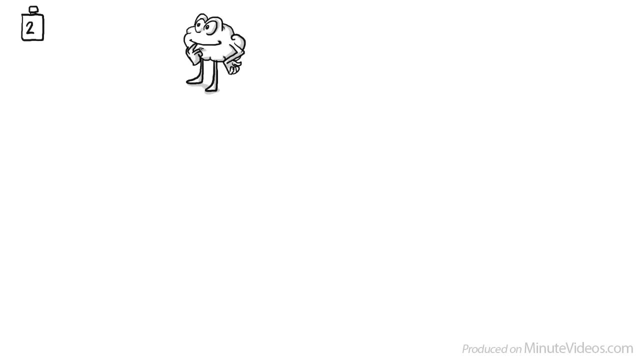 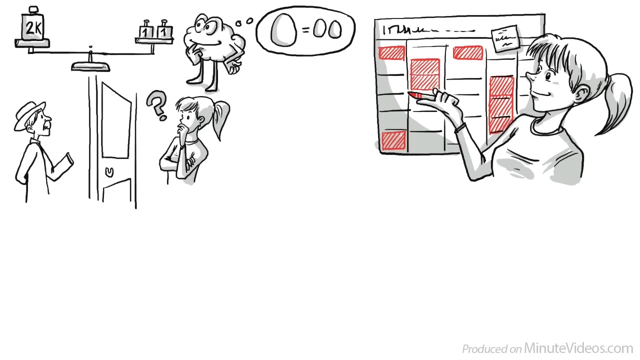 Our brain can now do deductive reasoning, which means we can compare two statements and reach a logical generalization. Our new mental skills allow us to plan our life systematically and prioritize, and we can make assumptions about events that have no necessary relation to reality. 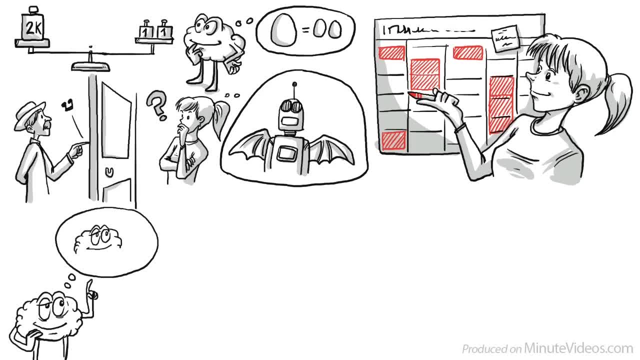 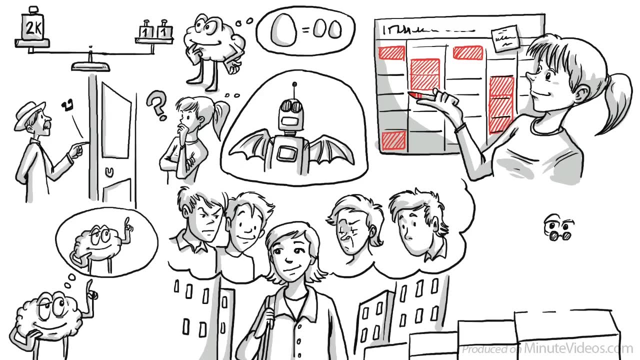 We can now also philosophize and just think about thinking itself. Our new sense for our identity now also creates egocentric thoughts, And some start to see an imaginary audience watching them all the time. Piaget believed in lifelong learning but insisted that the formal, operational stage is the final stage of our cognitive development. 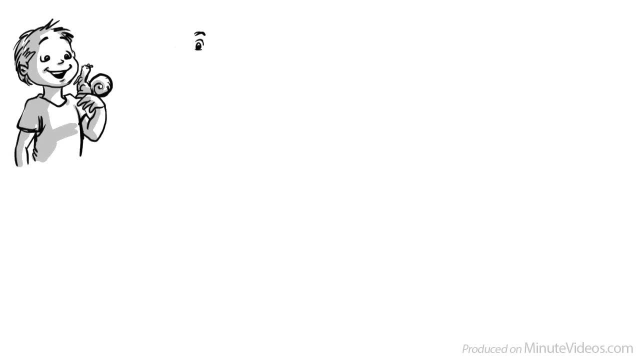 Jean Piaget's first interests were animals, and he published his first scientific paper on albino sparrows in 1907, when he was just 11 years old. In 1920, he began working on the first scientific paper on albino sparrows. In 1920, he began working on the first scientific paper on albino sparrows. in 1907,, when he was just 11 years old In 1920, he began working on the first scientific paper on albino sparrows.